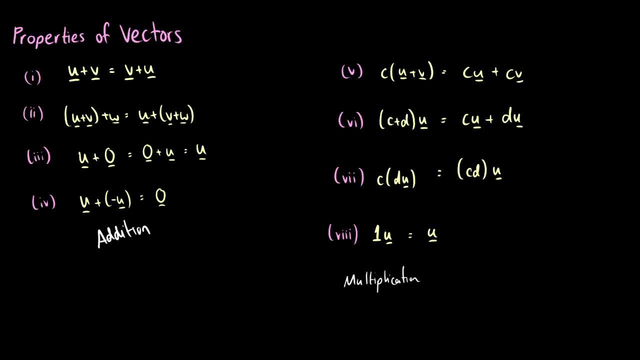 the last video with three u plus v is equal to three u plus three p. Number six says: if we take two scalars and we add them together and multiply by a vector, it's c times the vector plus d times the vector. Number seven says that we can multiply scalars first. And number eight says: if we multiply, 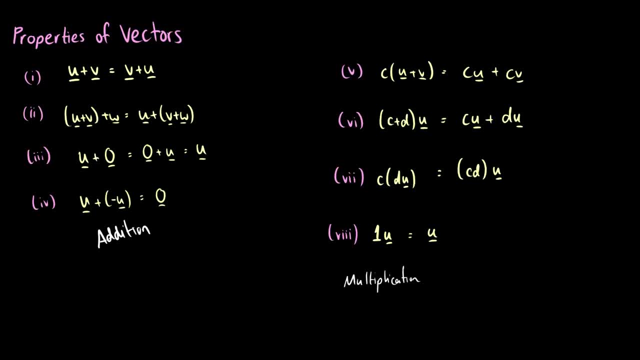 any vector by one, you get the same vector back. So we're going to prove some of these and this is more of a proof video. So we're going to prove that two vectors are the same, regardless of which order you add them. So what we say is we say that u one or, sorry, that u vector u. 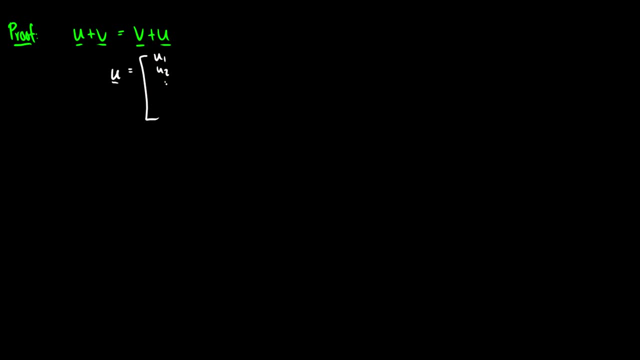 is a list of entries: u one, u two, all the way down to u n, and we say that v is the same thing And this will always be the same. So when we add these two together, we take u plus v. 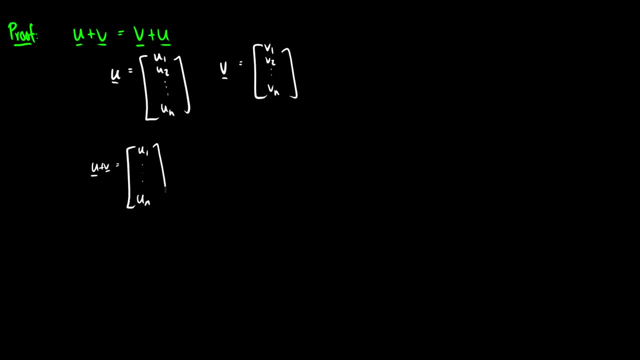 we take this list- u one down to u n and we add v one down to v n, So we know how to add these entries together. That means now we're going to be able to multiply by a vector and we're going to 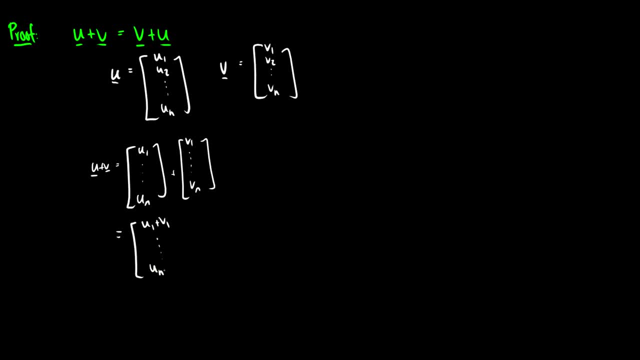 get v one and we're going to get v? n. So now we take u one plus v one and that goes all the way down to u? n plus v n, And we can switch the order of this thanks to the properties of real numbers. 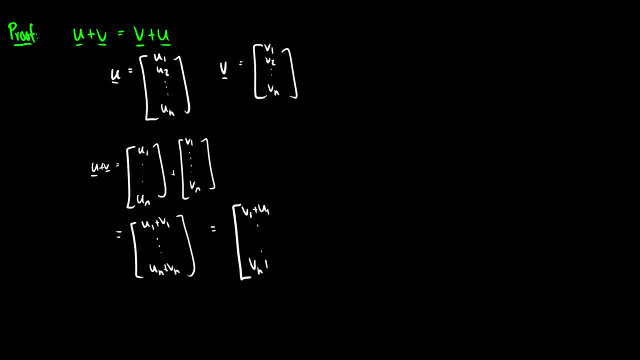 We know when we do real numbers we can switch the order. So we can say this is v one plus u one all the way down to v n plus u n, And that means that we can break it back apart. So we know this. 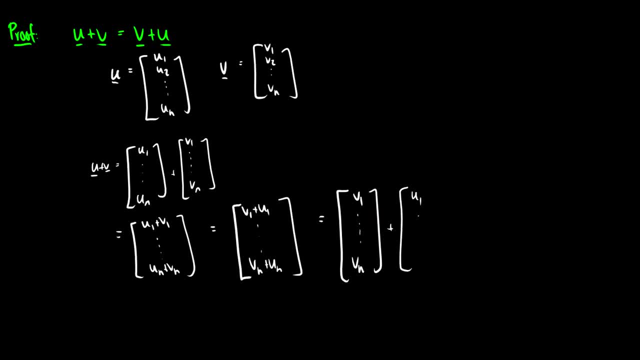 is the same thing as v one all the way down to v n plus all the way down to u n. So we know, this is just the same thing as v plus u. So that is a proof that u plus v is v plus u. And you're saying: why do we have to do all this? 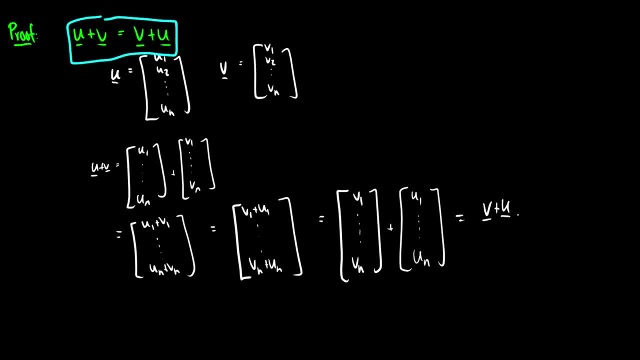 Well, we have to do this because vectors are not real numbers. Vectors have a magnitude and a direction. So we've defined how we write our vectors. we've defined how we can add the two together and using the commutative properties of real numbers, 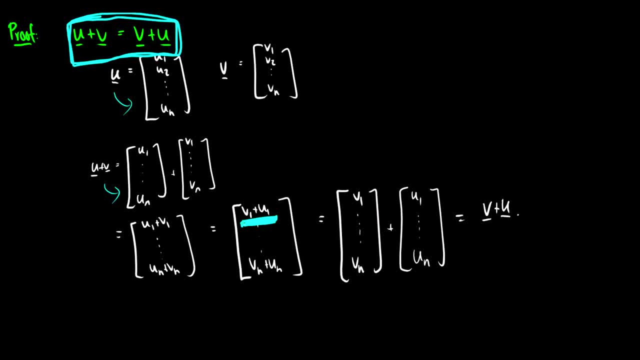 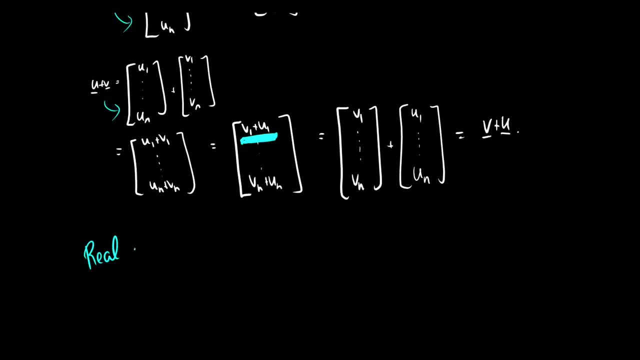 we have established a commutative property of vectors, So the real numbers establish vectors Or sorry, the properties of vectors. So we can't just assume that these properties of vectors are true. We now have a proof that this is true, So it might seem a little bit weird to do. 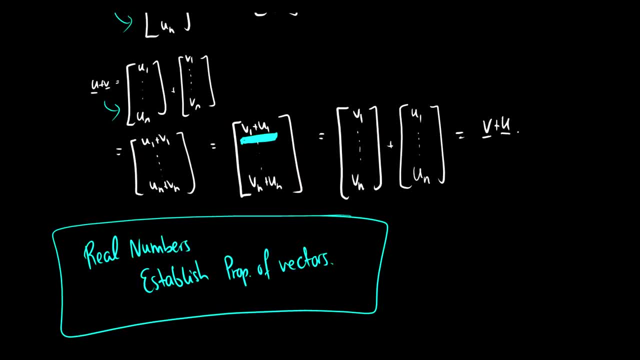 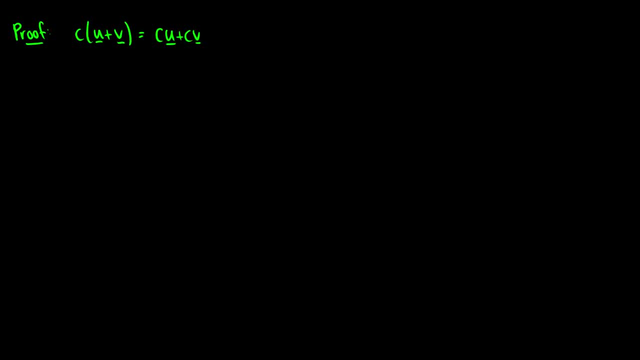 do it. but if you can do these basic proofs, you're in a good spot, because you understand how vectors work. Here's another one. If we have a scalar times u plus v, then we get a scalar times u plus a scalar times v. So again, we denote u plus v the same way. So here's what we do. We take 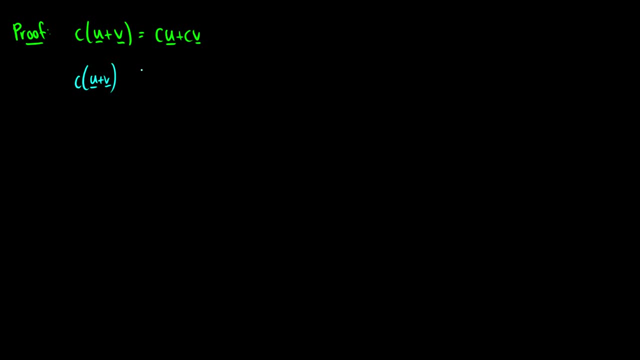 c times u plus v. So here's what this is. This is a scalar times u1 all the way down to un plus v1 all the way down to vn. So now we can distribute our scalar in there, So we can say: okay, this is actually the same thing as 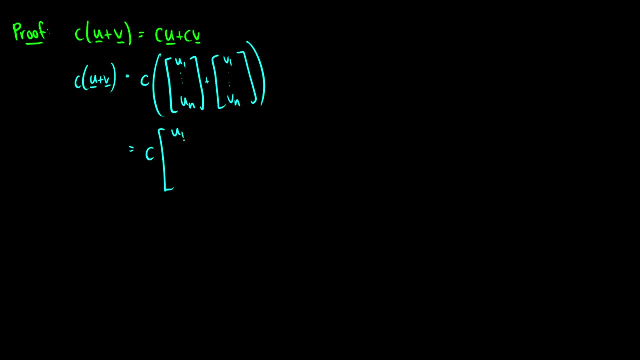 c times u1 all the way down to vn. So now we can distribute our scalar in there, So we can say: this is a scalar times v1 all the way down to un, plus v1 all the way down to vn. Sorry, this should be plus and I should have the c in there. So let's move this over. That does not. 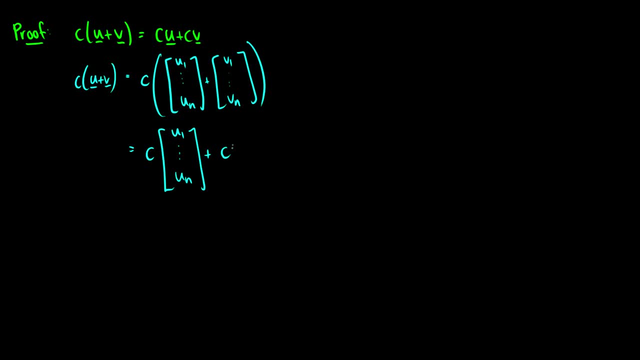 want to move over at all. So this is plus c times v1 all the way down to vn, And we know that this is just c times v1 all the way down to vn. So we can say, okay, this is a scalar times u1, all the. 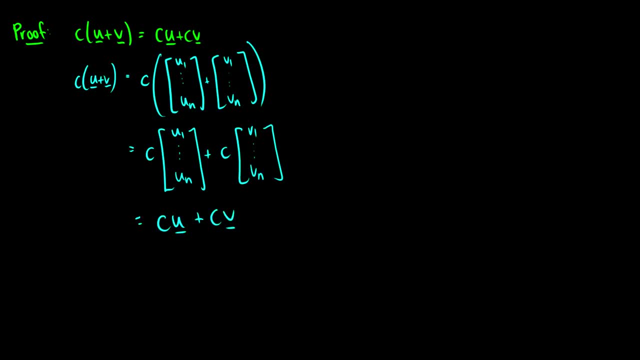 C times U plus C times V. So we have shown that this is true. You could go one step further and you could say: this is equal to CU1 all the way down to CU2, or, sorry, CUN plus CV1 all the way down to CVN. 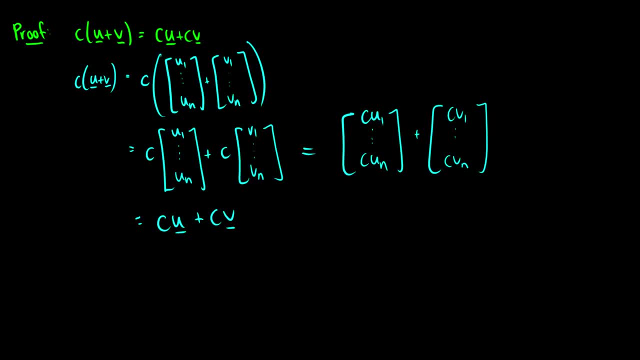 And that could be your final step, but that's not necessary. So there's a proof that that works. So those are two proofs right there. We'll do one final proof. We're going to show that a vector- U plus negative U, is equal to the zero vector. 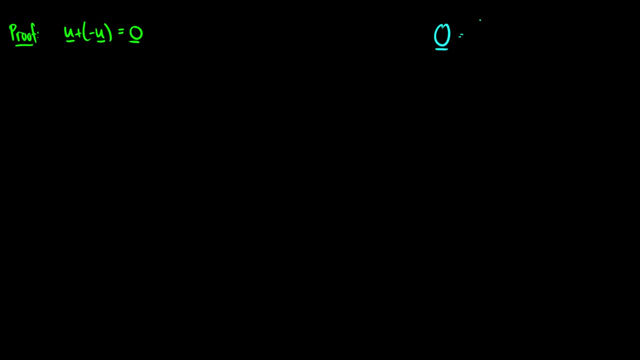 So what do I mean when I say zero? with a line under it? That means that each entry in the vector U or the vector zero is just zero. So what does this look like on a graph? It looks like that. 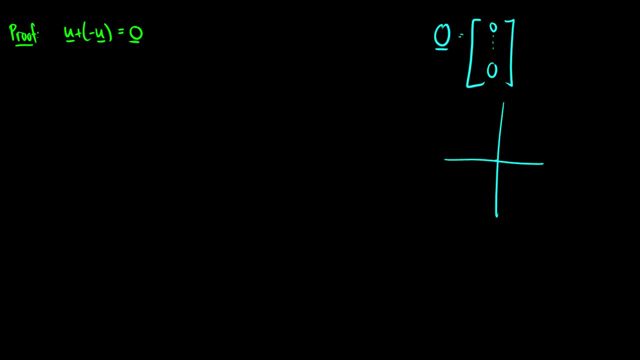 There is no vector, It's just zero. It stays at the origin. So let's prove this. So let's start with the vector U plus negative vector U, So this is equal to U1 all the way down to UN. 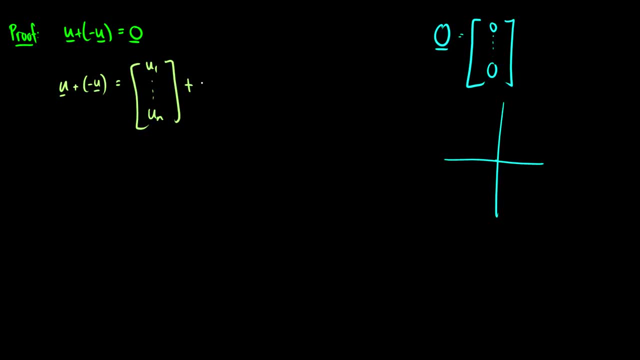 And then we say it's plus negative U1 all the way down to negative UN. So let's add these together So this is U1. So this is U1 minus U1, all the way down to UN minus UN. 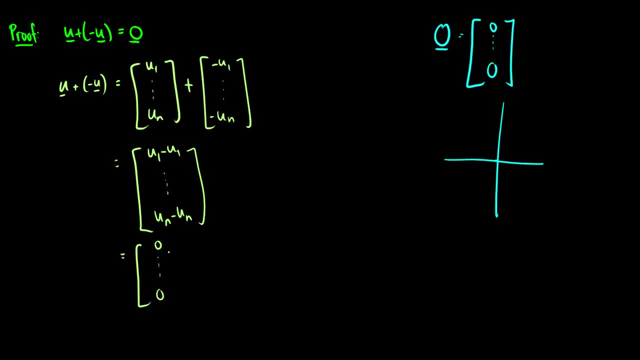 And this is just equal to zero, all the way down to zero, which is just the zero vector. So we've proven those properties. So those are three of the eight properties that we have proven, And I challenge you to prove the rest of these. 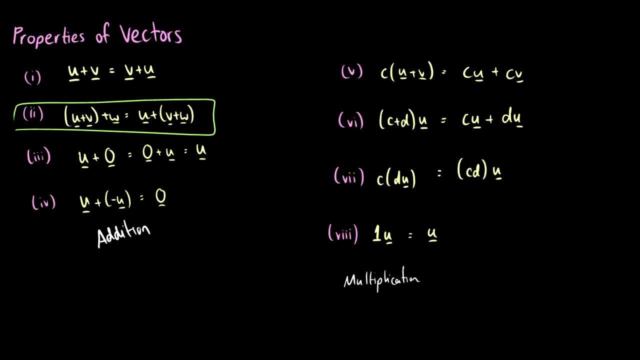 Prove number two. Number three is very, very easy. Number four, Number six is probably good to prove. Number seven is good to prove. Number eight does not really need proving. So I challenge you to try to prove these three on your own. 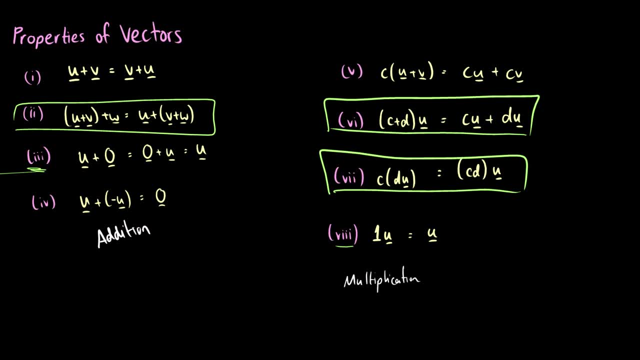 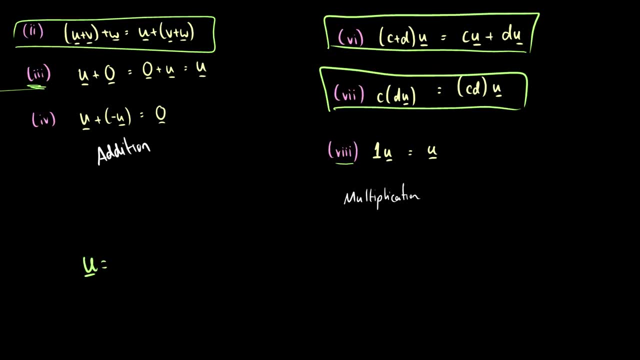 You can give them a shot in the comments below and I'll tell you if they're right or not. If you want to prove them more nicely in notation, it is perfectly okay to say that the vector U is equal to this ordered list and all the way up to UN. 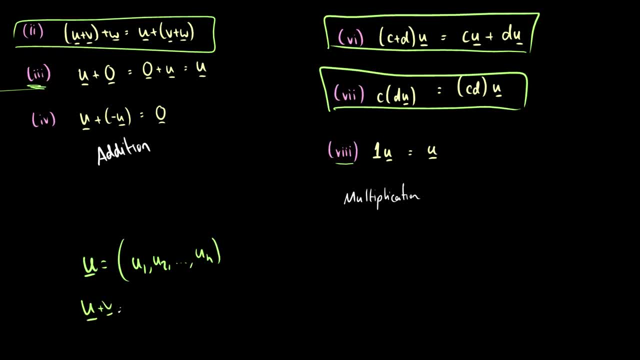 And then you could say, for instance, that U plus V Is just U1 plus V1, comma, all the way up to UN plus VN comma, And that is perfectly okay when writing out proofs as well. So give those a shot and hopefully you'll get them right.